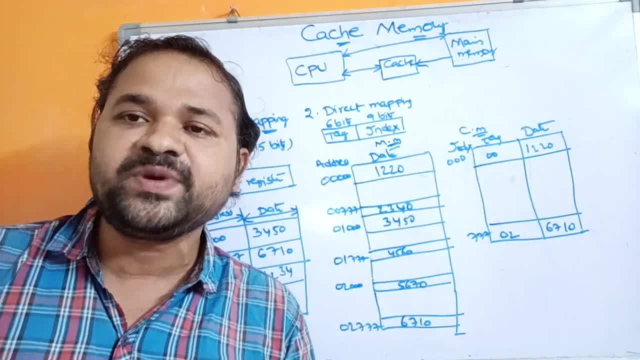 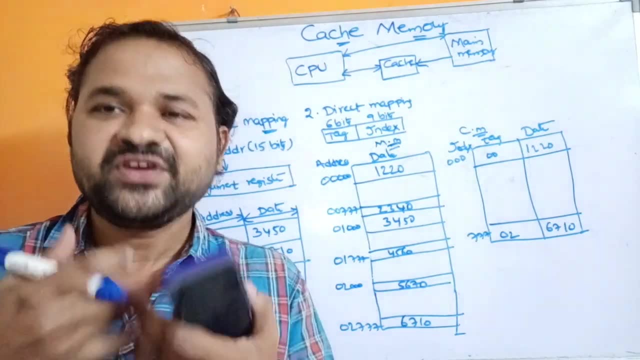 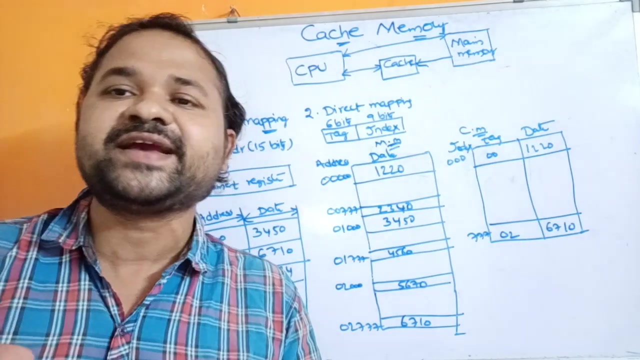 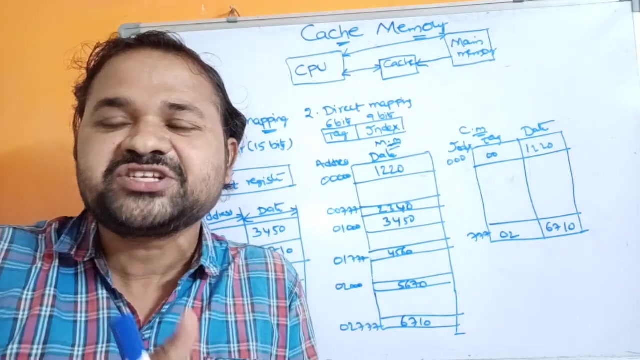 Whereas the remaining statements are to be executed only once. Let us assume that we have a program which contains function calls. We know the advantage of the functions. Functions are mainly useful for reusability purpose. So that means if we want to execute a set of statements repeatedly, then only we use the function. So that means here we may call that function several times, So that function call will be executed several times. 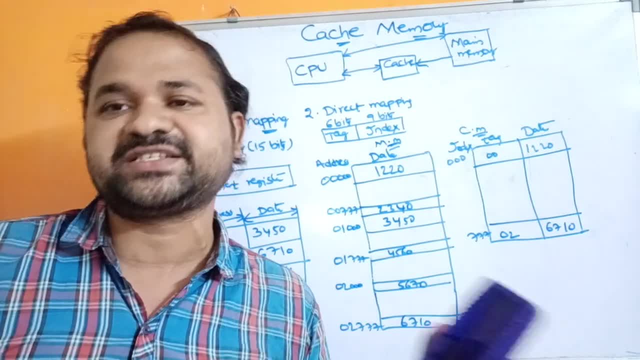 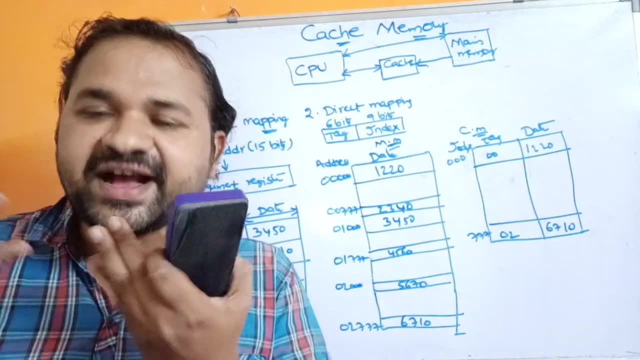 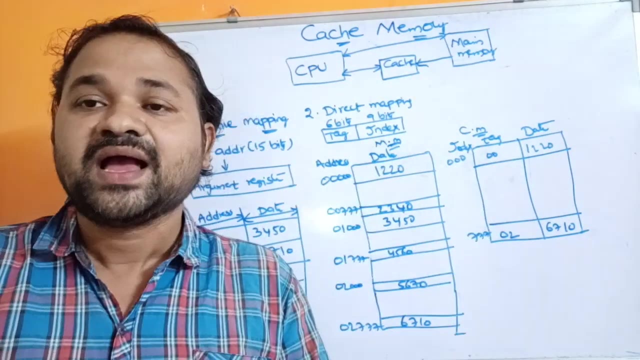 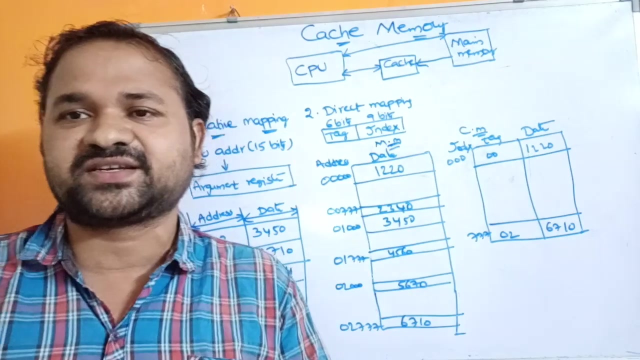 And the remaining statements are to be executed only once. So here the point is: if a program contains some looping control statements or function calls, then those statements are to be executed very frequently, very repeatedly, and remaining set of statements are executed less frequently. They may be executed only once. This property is called as locality of reference. 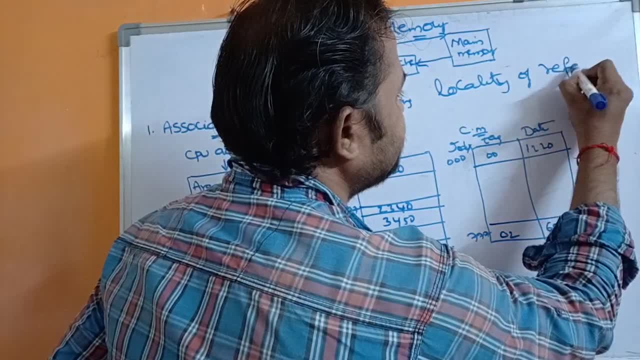 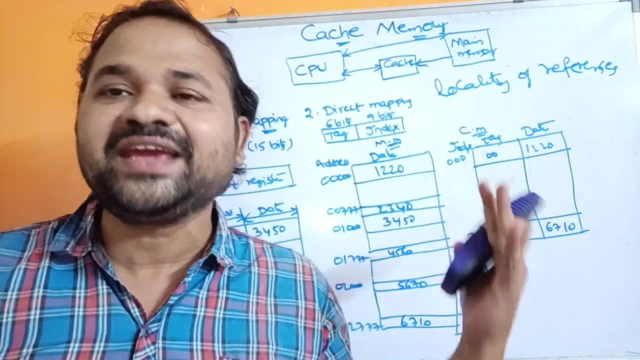 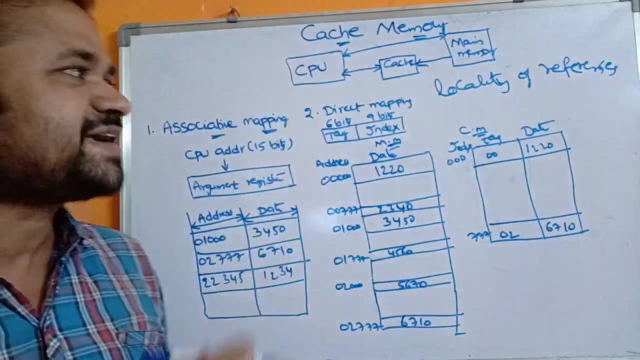 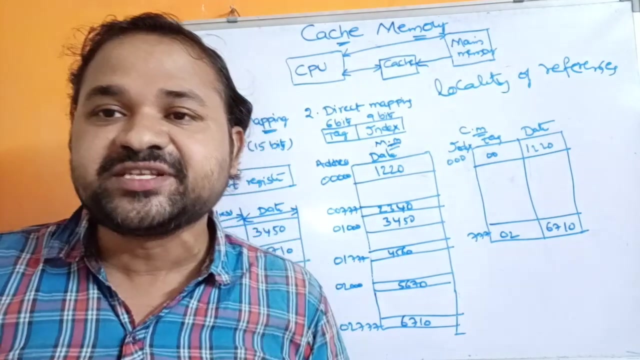 So locality of reference states that a certain set of statements are to be executed very frequently and the remaining statements are executed less frequently. So now, with the help of the catch memory, what we can do is if we place those active instructions, those frequently used instructions, those repeatedly accessed instructions, in the catch memory. 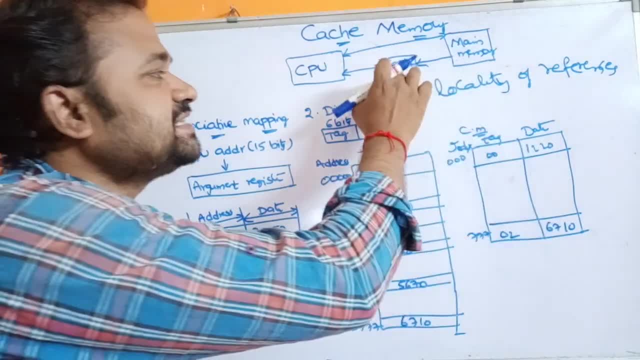 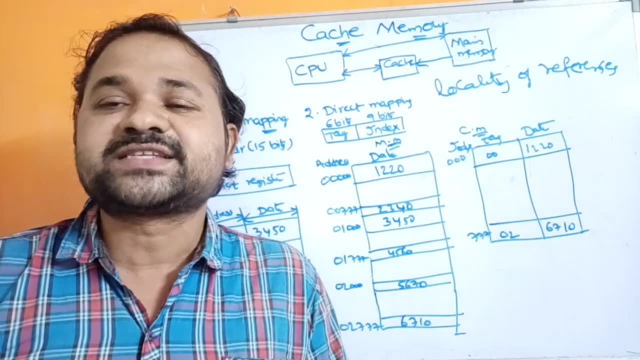 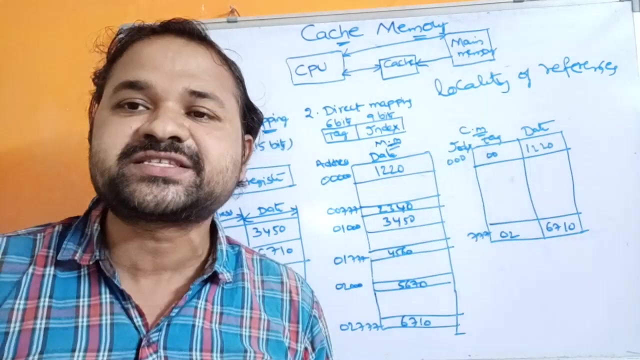 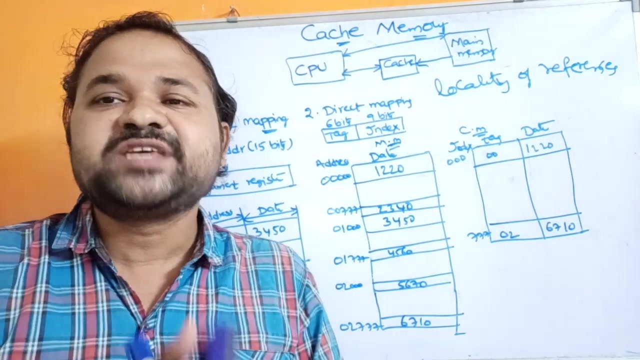 So if we place those frequently accessed instructions in the catch memory, then the total execution time of the program will be reduced. That is the average memory access time will be reduced Why? Because the advantage of the catch memory is catch memory access time is extremely faster than main memory access time, So CPU can access the content of the catch memory very, very fastly. the total execution time of the program will be reduced as well as the average. the total average memory access time will also be reduced. so that is the advantage of the cache memory. so that's why we have to place the cache memory in between CPU and main memory, so whenever CPU needs to execute an instruction or 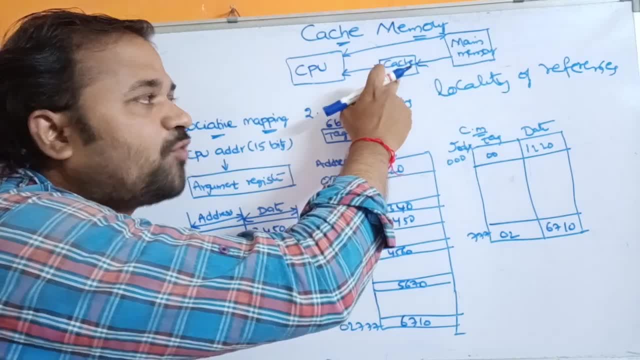 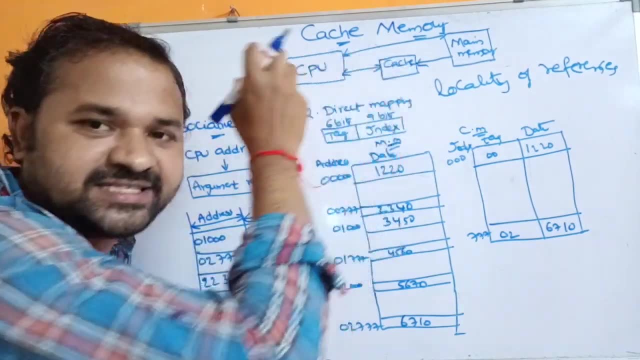 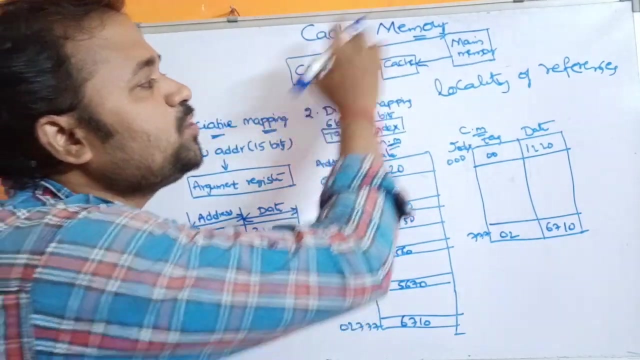 a word, then first it checks whether that word is present in cache memory or not. suppose if the word is present in cache memory, then CPU access that word and executes that word. suppose if the word is not found in the cache, then CPU access the main memory, so from the main memory that word will be transferred to. 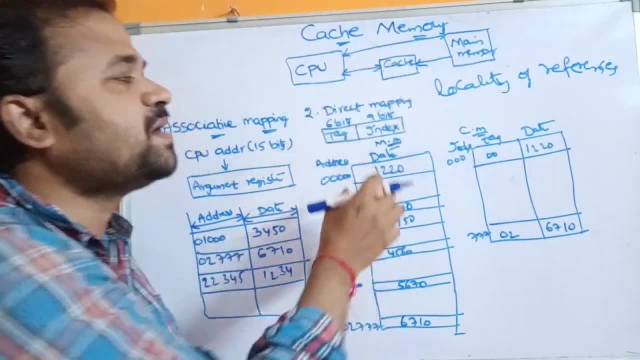 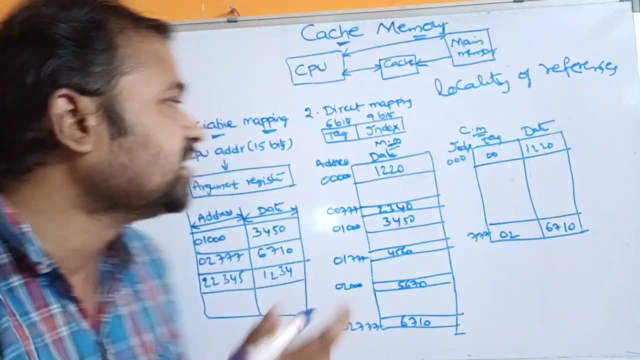 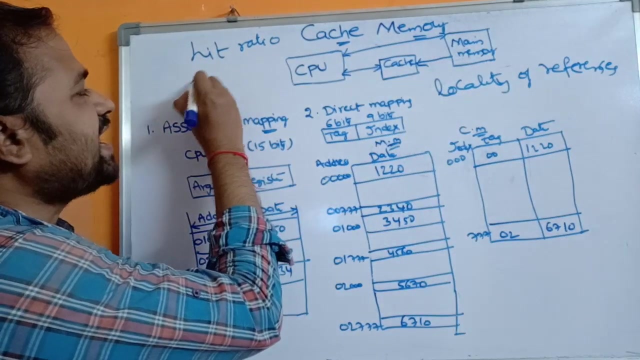 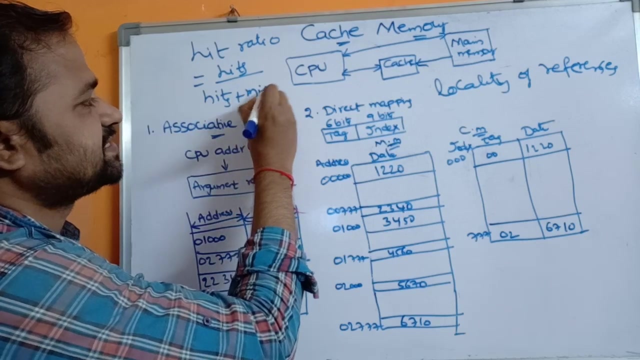 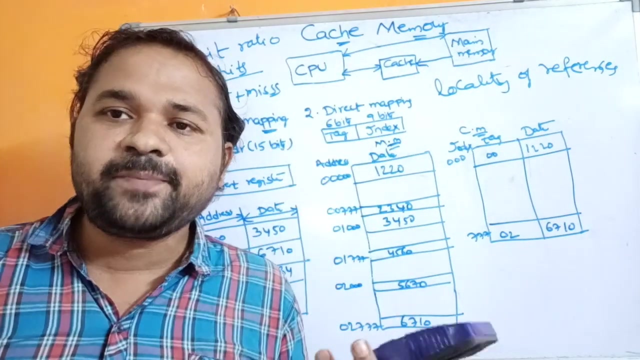 the cache memory. so now CPU access the cache memory to execute that word. okay, here we can analyze the performance of the cache memory by using hit ratio. okay, here we have hit ratio, hit ratio. we can calculate the hit ratio with the help of the formula called number of hits, by hits and misses. hits and misses, so this: 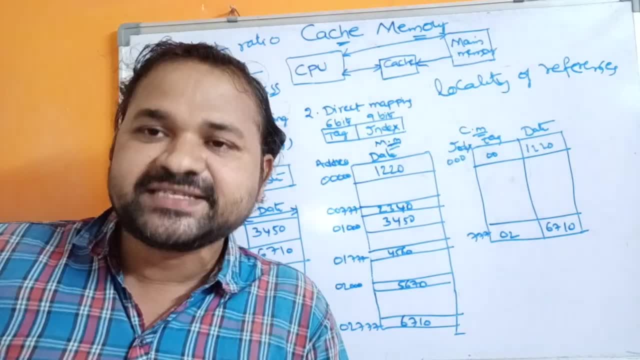 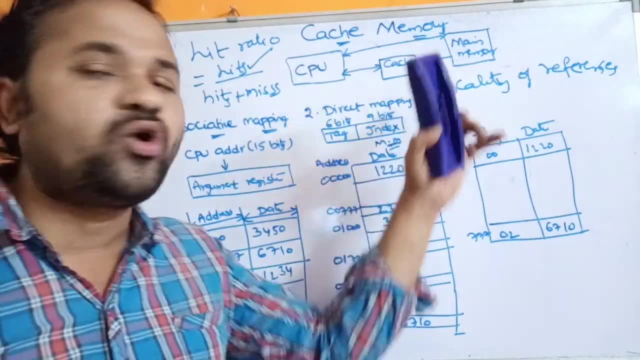 is the formula for hit ratio. hit means whenever CPU needs to execute a vote, it checks whether that vote is present in the cache or not. suppose if the vote is. if the word is not present in the cache, then cpu access the main memory. so if the word is not, 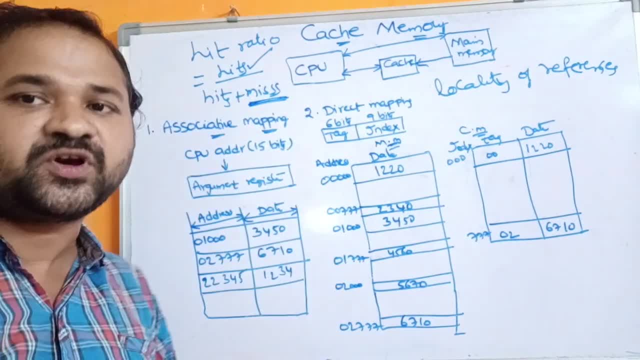 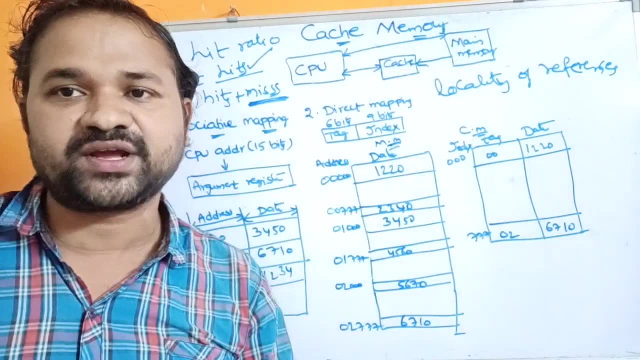 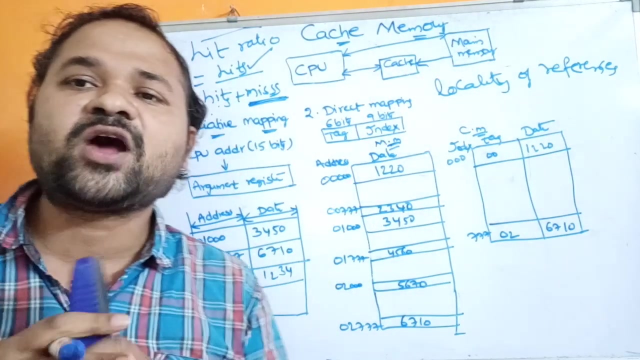 present in the cache. then it is called as miss. okay, so that that word should be transferred from main memory to the cache memory. so cpu access that word, okay. so the formula here is the formula for hit ratio is number of hits by number of hits plus number of misses. so as a user, as a developer, 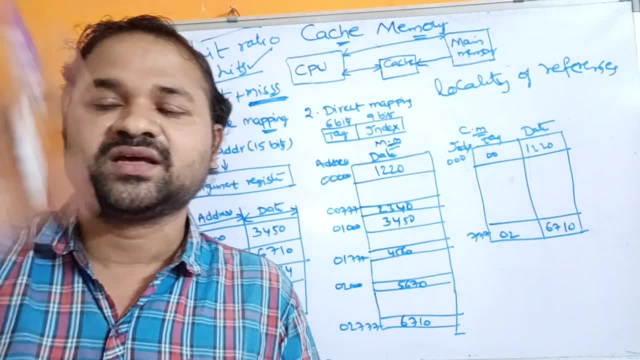 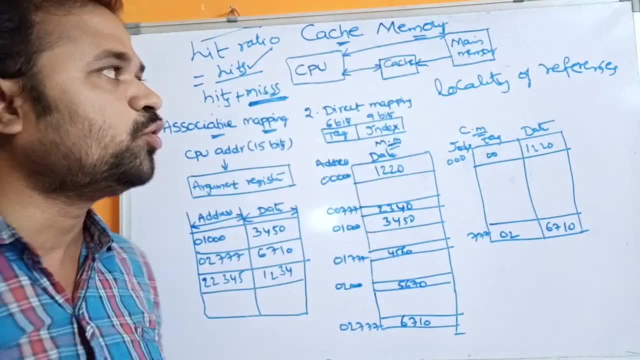 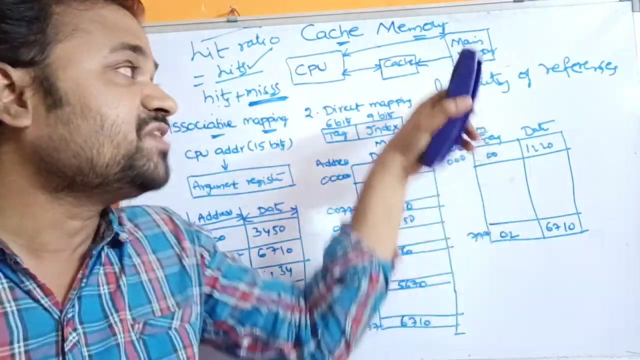 our target should be. hit ratio will be very, very high. so hit ratio will be very, very high means most of the time cpu is accessing cache memory instead of main memory so that with less amount of time we can execute the program here. if the vote is not present in the cache, then the 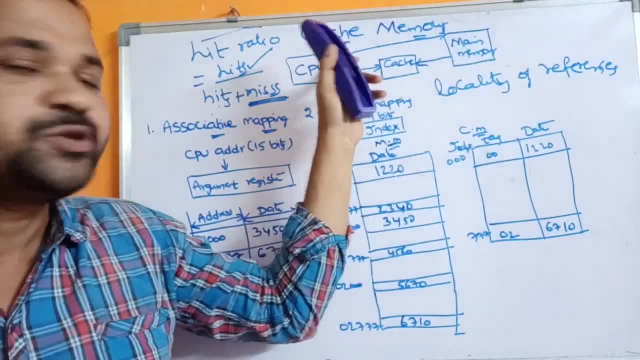 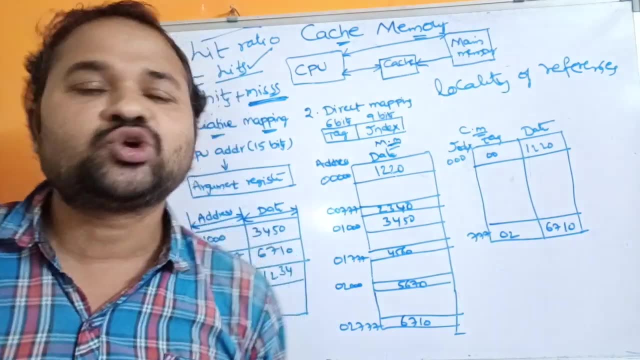 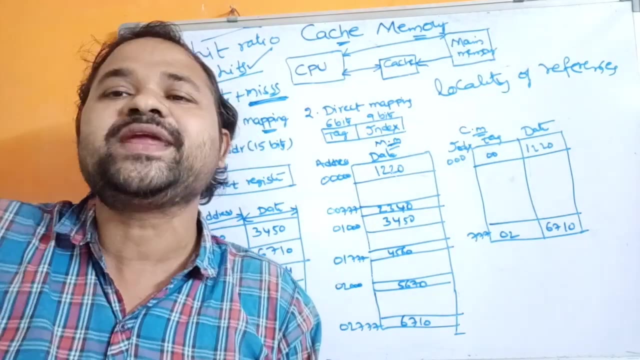 corresponding board should be transferred from main memory to the c main memory- i'm sorry, main memory to the cache memory. so how the transformation will be done? so that should be done with the help of mapping. so mapping is a process by using which the corresponding board will be transferred from main memory to the cache memory. here, mainly, there are: 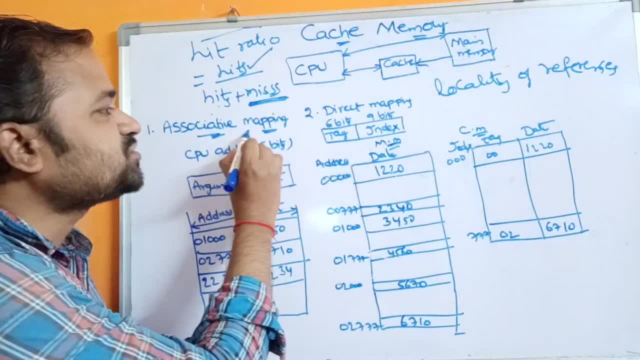 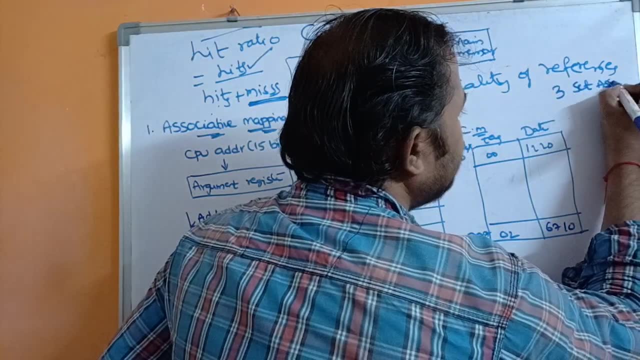 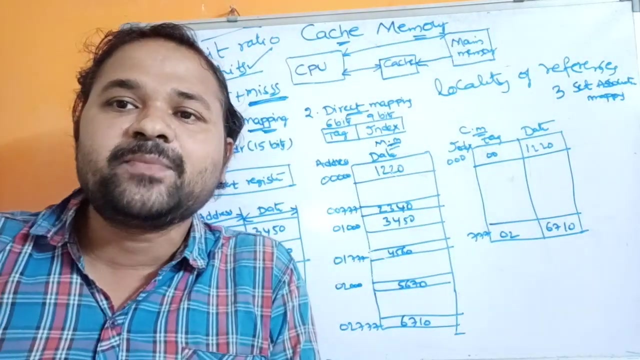 three types of mappings are available. the first one is associative mapping. second one is direct mapping. third one is set associative mapping. associative mapping, direct mapping, set associative mapping. so by using mapping we can transfer the code to the cache memory and we can transfer the vote from main memory to the cache memory. so first let's see about associative mapping. 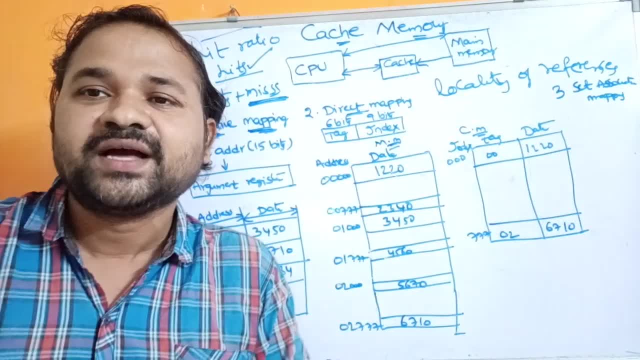 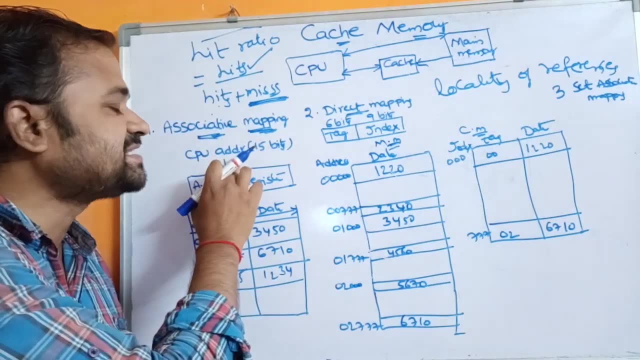 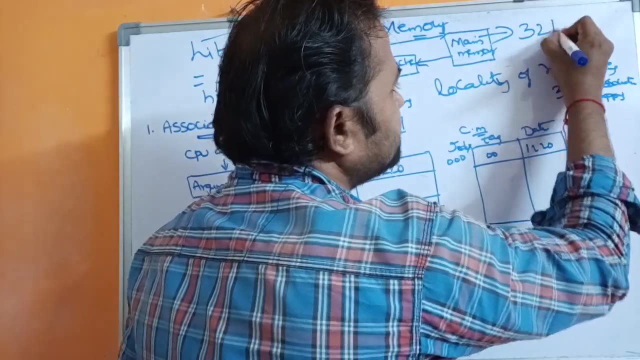 why this is namely as associated associative mapping means. here we are in order to implement the cache. we are using some associative memory here here, cpu generated your address here. here the address size is 15, 15 bits. here here, the size of the main memory is 32k votes. 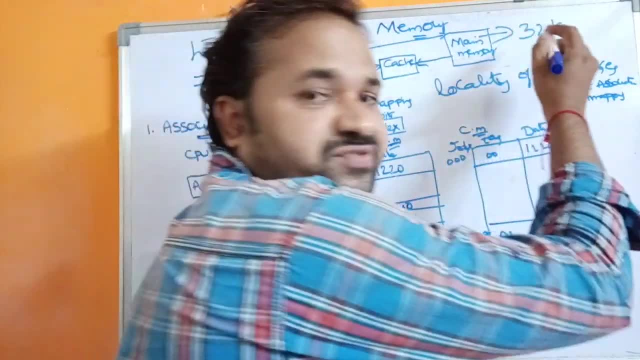 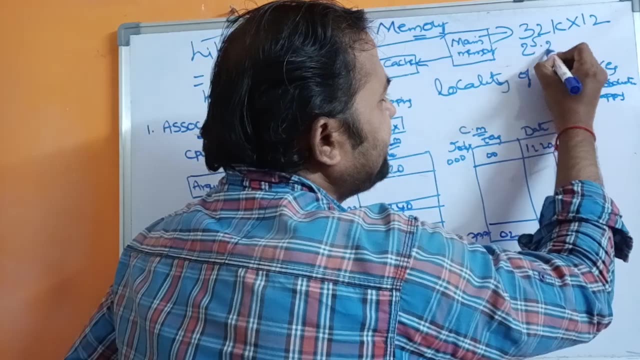 let the size of the main memory is 32k votes, where each vote store 12 bits of information. here 32 k means 32 means 2 power 5. 1 kilobyte is nothing but 2 power 10.. so 2 power 5 into 2 power. 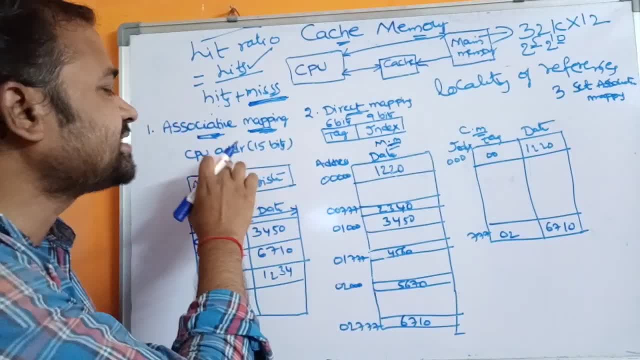 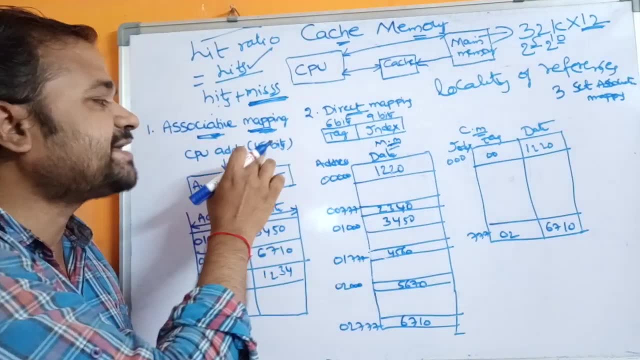 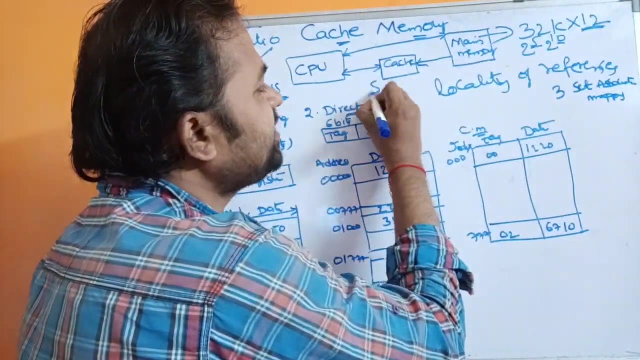 10 is nothing but 2 power 15. so here the cpu address size is 15 bits where each vote contains how many bits? 12 bits, okay, so the data size is 12 bits. so address size is 15 bits where he has data sizes: 12 bits. so out of those 32k boards a cache memory can store data game. it can store 512 votes. 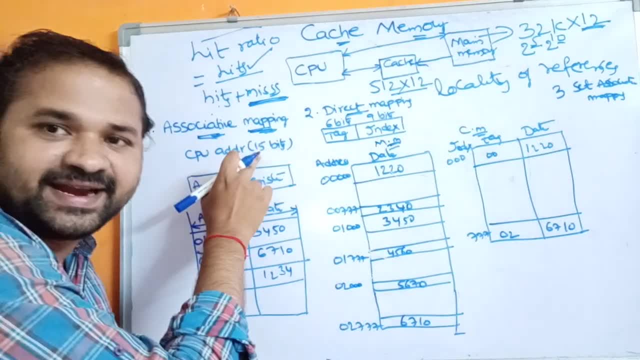 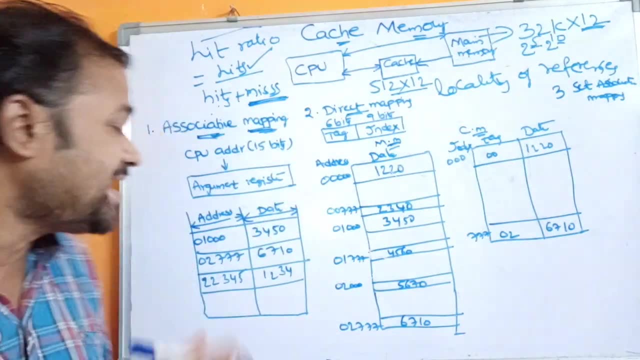 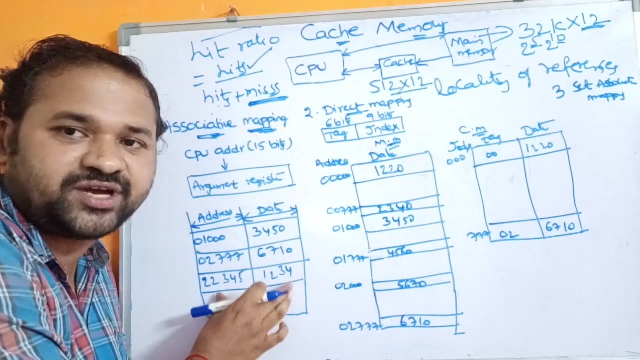 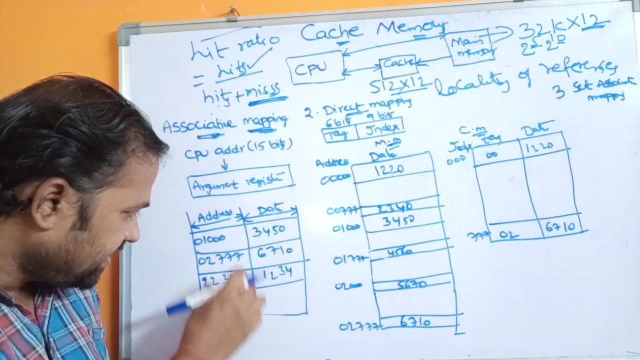 at one pitch. okay here. cpu generated an address. address size is 15 bits. that corresponding address will be stored in argument register. then the address of the argument register will be compared with cache memory. so this is nothing but associated to memory cache. okay, associated mapping catch. associated mapping catch. okay here. uh, here, with the help of this memory, we are storing three. 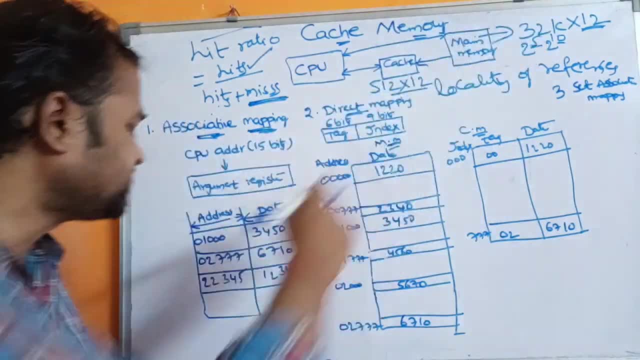 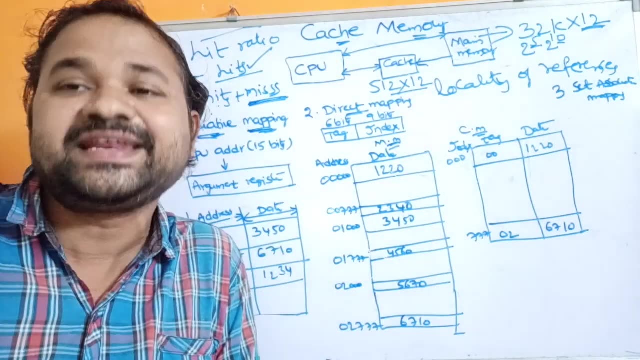 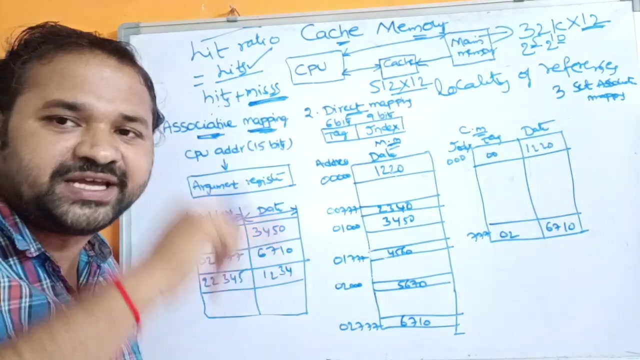 votes here. okay, where we know that each word address size is 15 bits, here we are using after notation. after notation means each digit represents three, three bits. each digit represents three bits of information. so here totally we have five digits, are there? so five into three, so that is nothing. 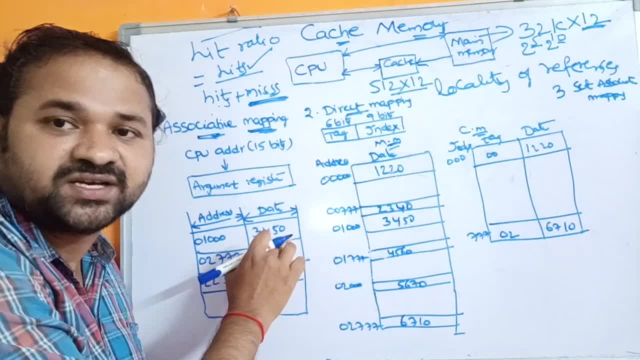 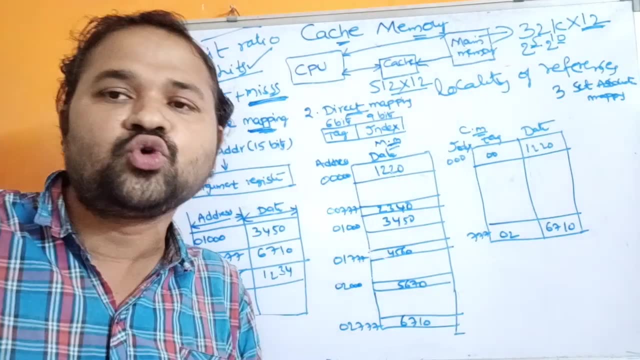 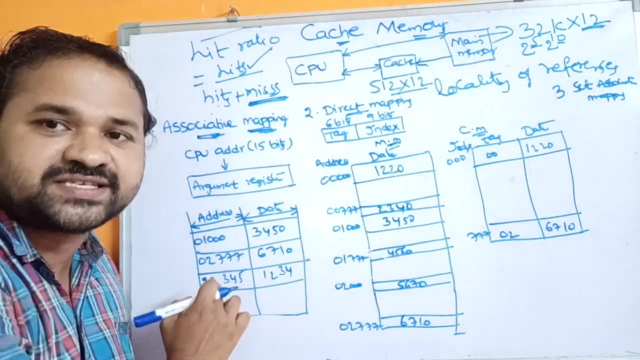 but 15 bits here. data size is what? 12 bits, four digits. so four digit means one digit is equal to three bits of information after representation. four, two, one. so So here the address of the argument register will be compared with address of this associative mapping catch. 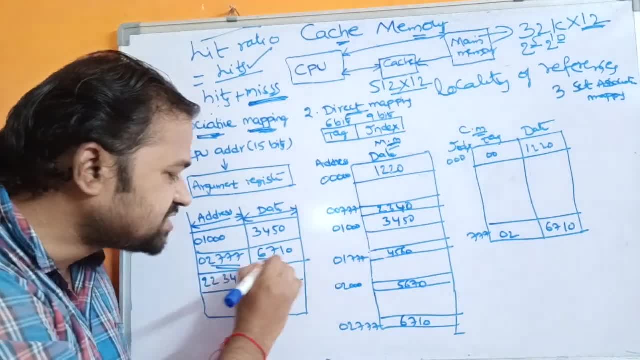 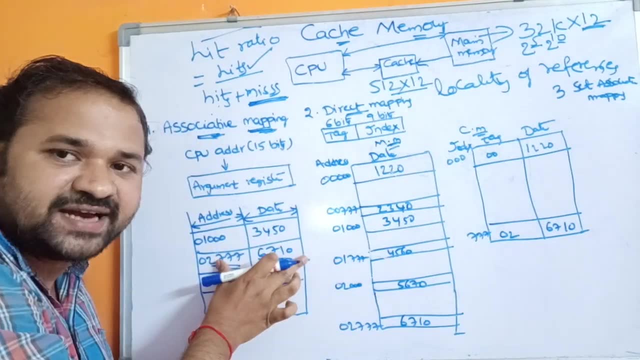 Let us assume that this is the corresponding address. So this word will be delivered to the catch. So catch memory will execute the word. So totally, there are three words. are there again? This is nothing but address of each word. This is nothing but data. 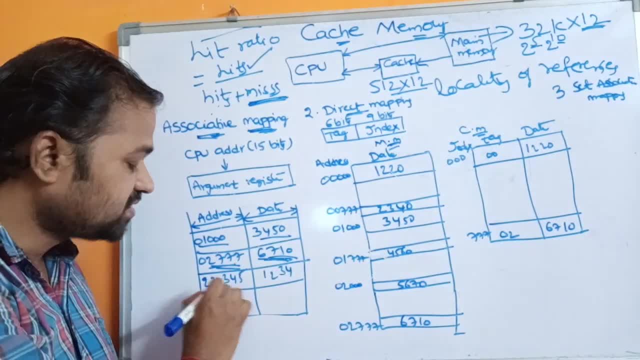 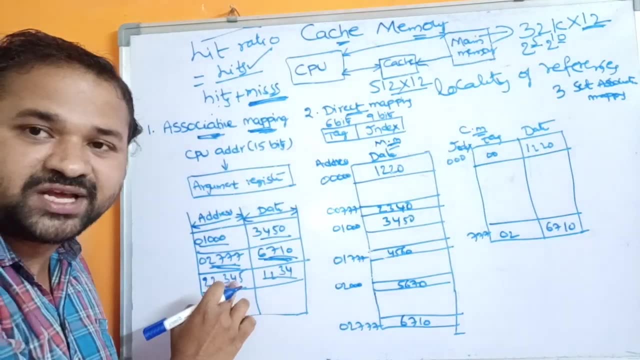 So first word address. first word data. second word address. second word data. third word address. third word data. like that, Next CPU generated an address called 22345. So here we have 22345. So this 22345 will be compared with all the addresses. 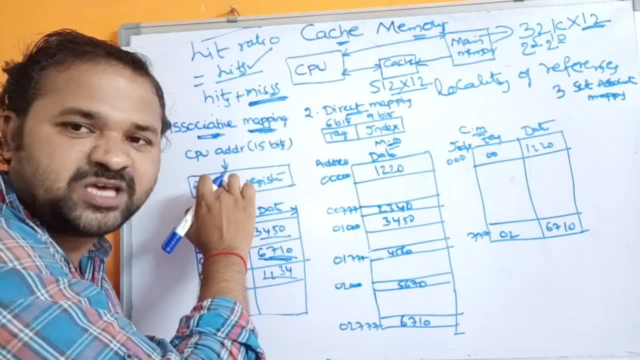 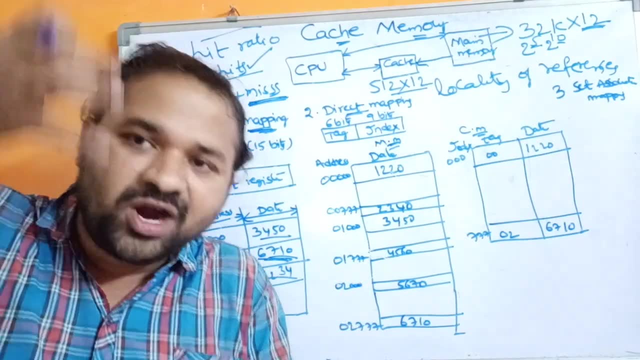 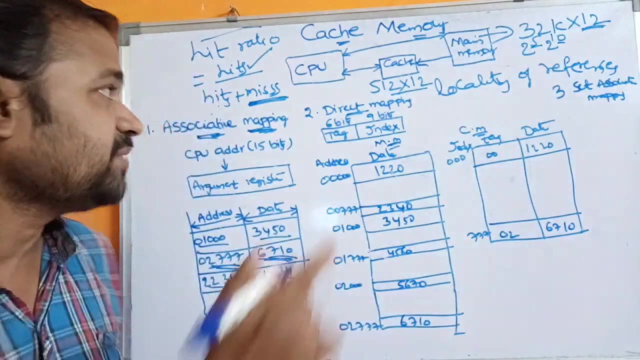 So here a match is found. So this word is delivered to the CPU. So CPU executes that word. Suppose, if the corresponding word is not present in the catch, then that word will be transferred from main memory to the catch memory. Let us assume that catch memory is completely full. 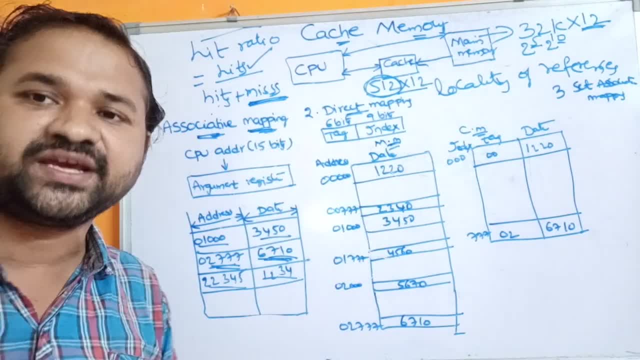 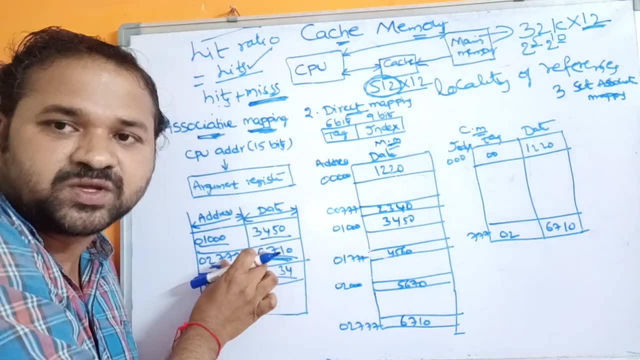 Why? because at a time the catch memory can store only 512 votes only. Let us assume that catch memory is completely full. Then we have to replace one of the word in the catch memory to store new word from the main memory. So which word we have to replace? 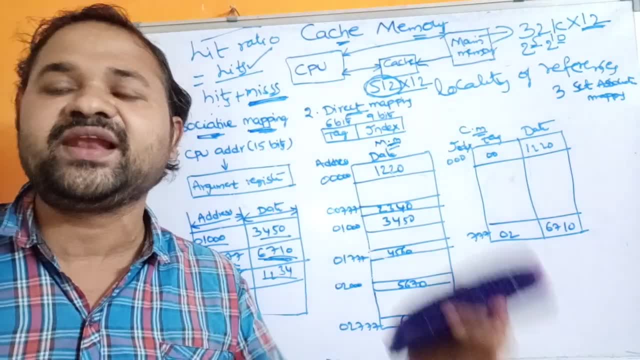 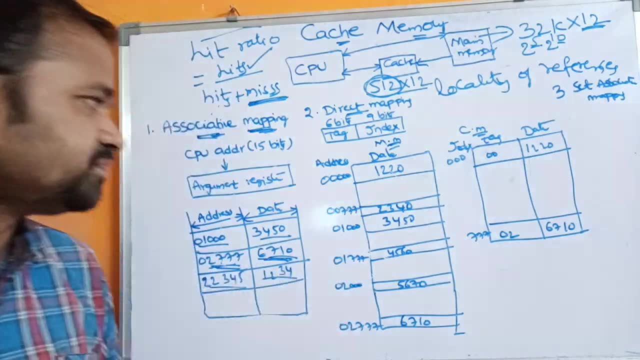 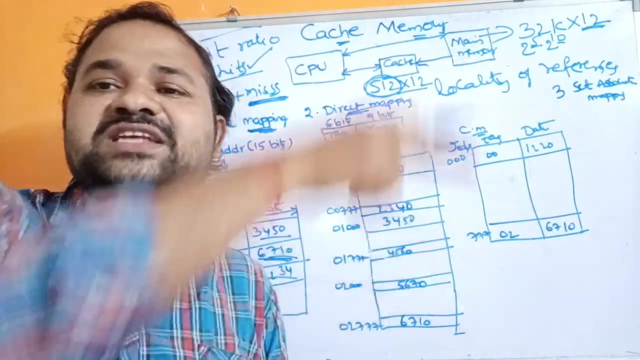 That depends upon the replacement algorithm we use. We have FIFO algorithm, OPT algorithm, LRU algorithm, So depends upon the replacement algorithm. we will replace the corresponding word. Now let's see about direct mapping. In direct mapping what will happen is that the CPU generated address is divided into two. 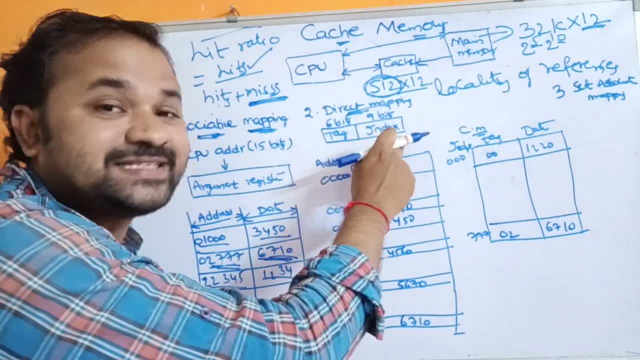 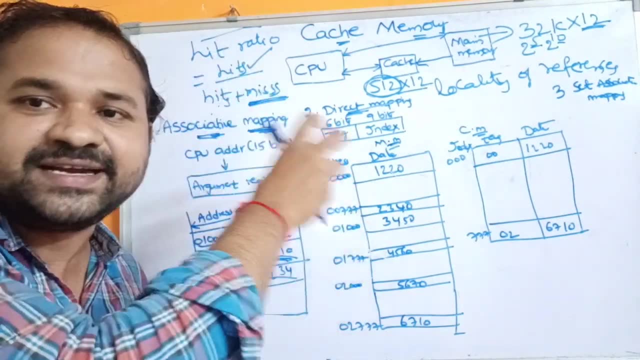 parts. The first part is tag address. The second part is index address. Here the size of the tag is 6 bits. So 6 bits means we need 2 digits for representing the data And the size of the index is 9 bits. 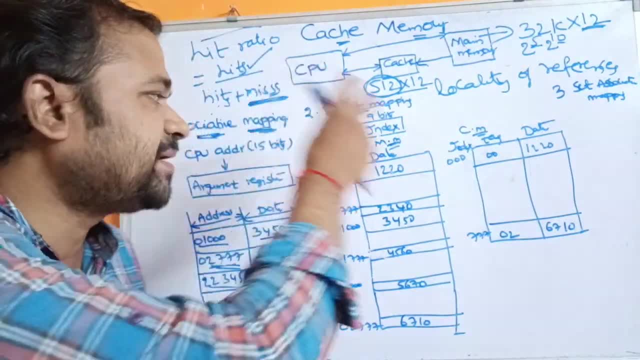 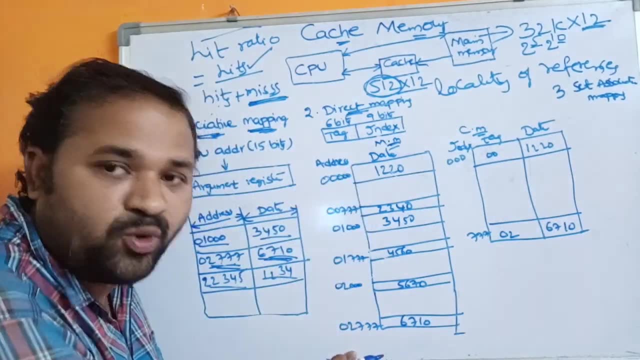 So 9 bits means we require 3 digits in order to represent that index address. So here we have main memory and here we have catch memory. So these are main memory addresses and these are nothing but main memory data. So 00000 is nothing but index address. 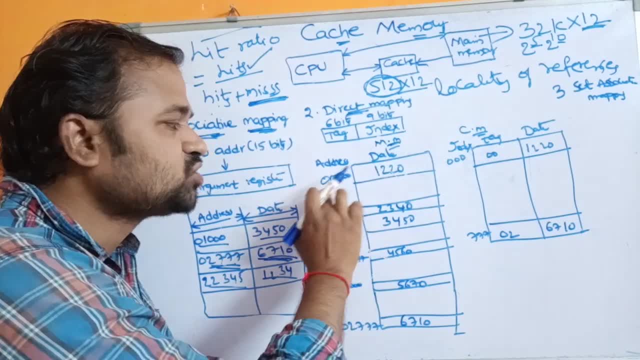 So here we have main memory and here we have catch memory. So 5 bits is nothing but address, 1220 is nothing but data. So 5 digits, 4 digits. So 5 x 3 means 15 bits, 4 x 3 means 12 bits. 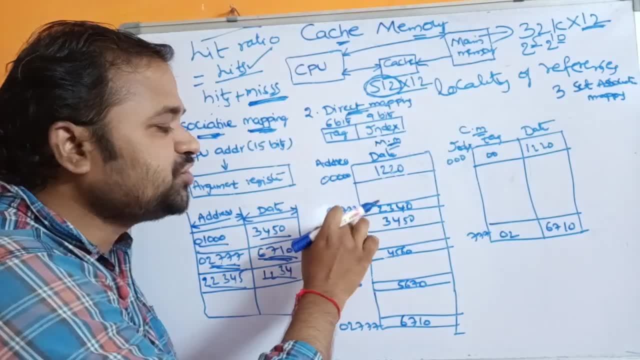 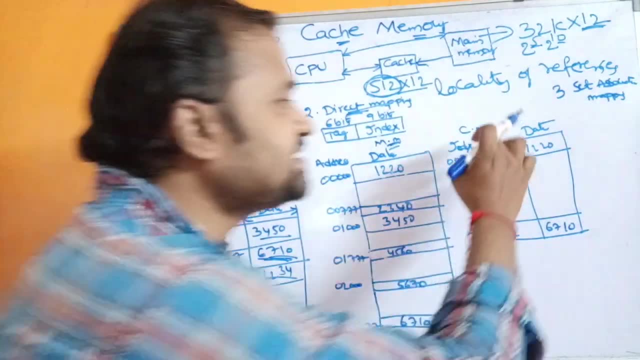 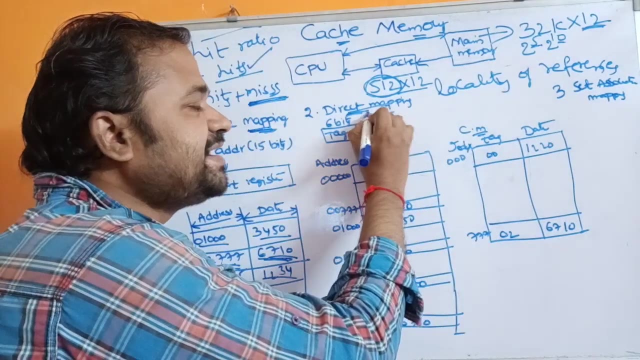 00777 means address. This is the data. So, likewise, we have taken some data in the main memory and this is nothing but the catch memory. In the catch memory, this is nothing but index address For representing the index address. index address size is 9 bits. 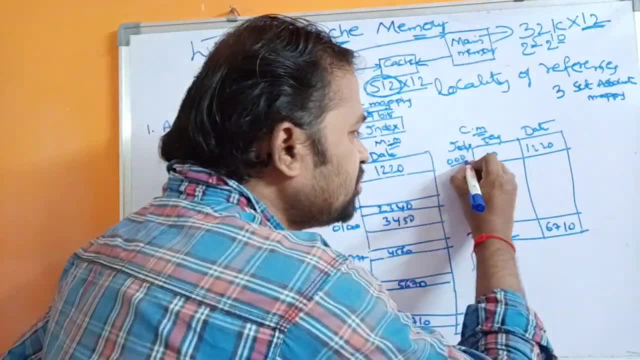 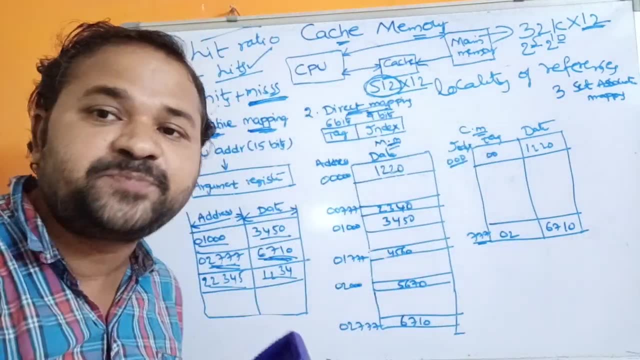 9 bits means we require 3 digits, So 000 is nothing but those 3 digits. Next, 000 is nothing but those 3 digits. Here tag means 6 bits. 6 bits means we require 2 digits, So 00 is nothing but those 2 digits. 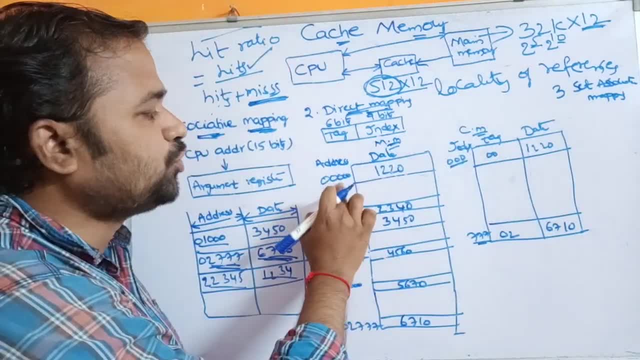 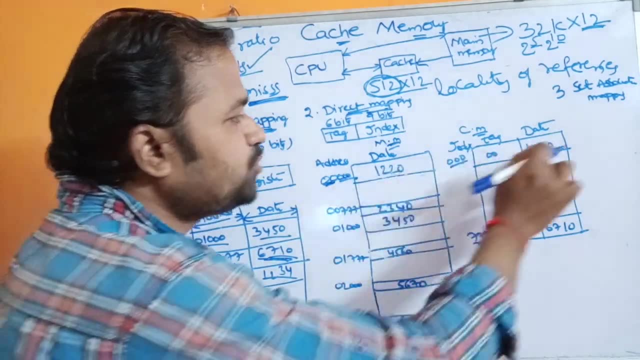 1220 means what Data Here? 000 means in 000,. first two zeros are nothing but tag, Next three zeros are nothing but index. 1220 is nothing but data In 02, this 02 is nothing but tag. 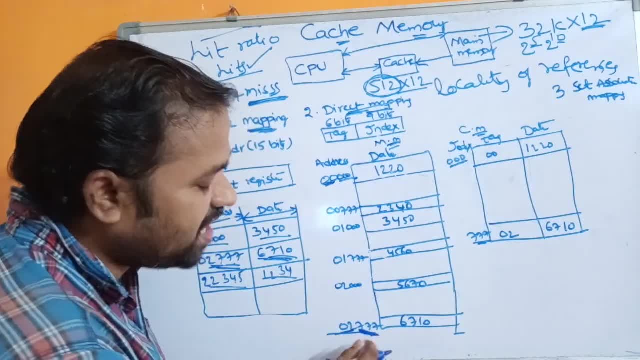 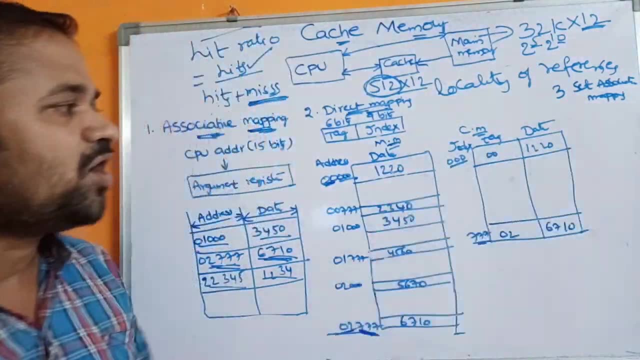 So the last 3.. So the last three digits are useful in order to access the index of the cache memory. So 6710 is nothing but data of the corresponding vote. Let us assume that CPU generated an address card 0 to 777. 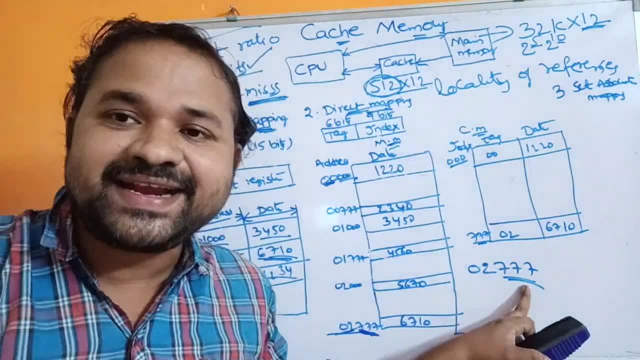 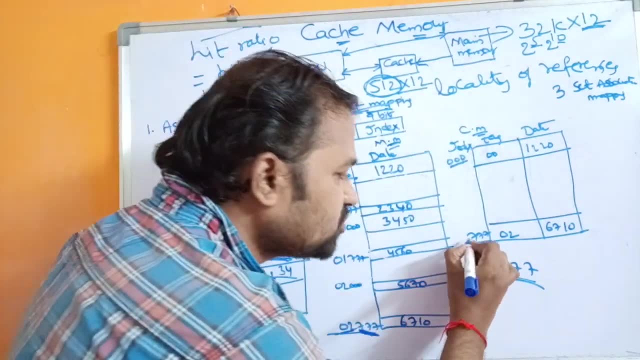 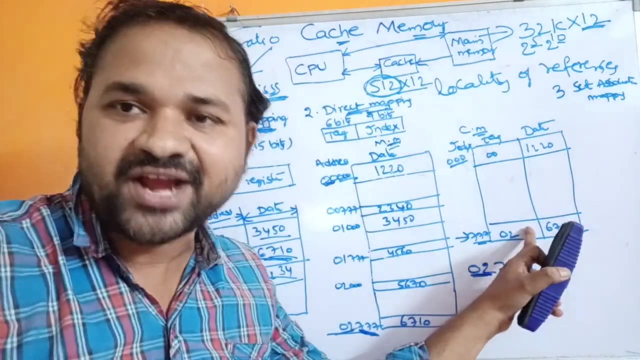 So then here this index address is useful in order to access the cache memory. So where the 777 is there in the cache memory. So this is nothing but the 777. Then after that we have to check whether 0 to E is tag or not. 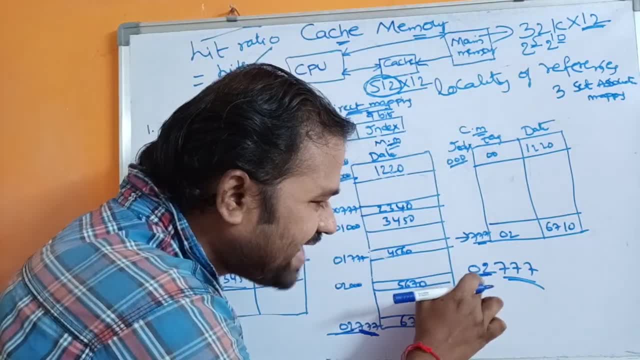 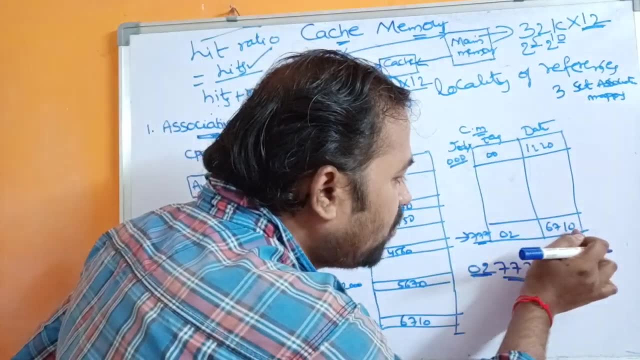 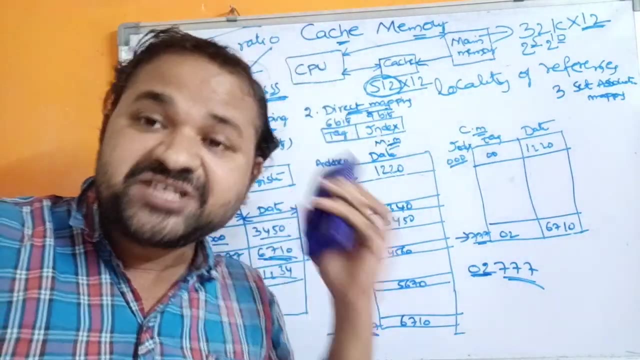 So we have to compare the CPU generated tag address with the cache memory tag address. If these two are same, then this vote cache memory will allocate this vote to the CPU. So CPU executes this vote. The major problem with this approach is if two are more votes with same index address. 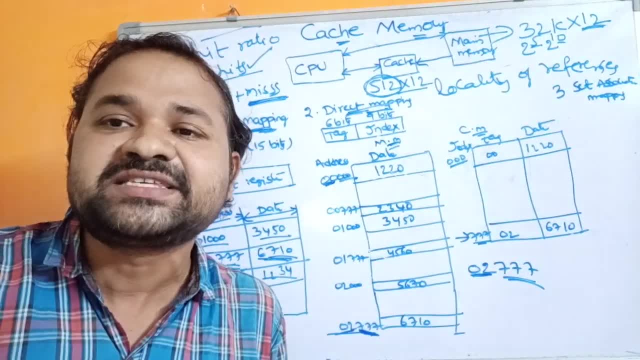 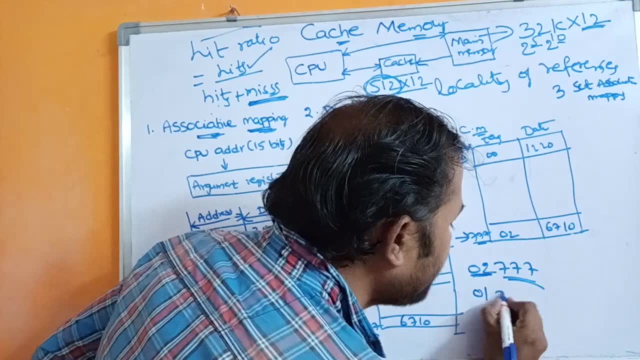 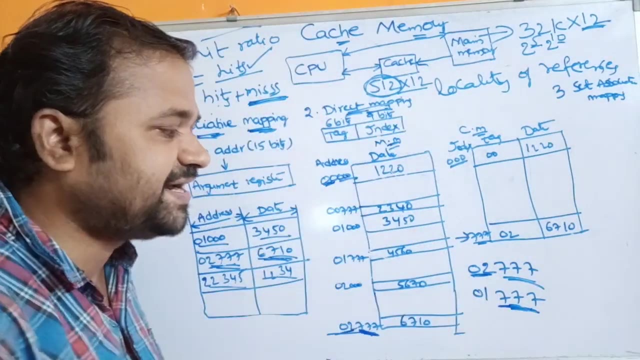 but with different tags or access it repeatedly, then hit ratio performance will decrease drastically. Let us assume that I want to access 0,, 1,, 777.. So in this, what is the index address? 777 is the index address. 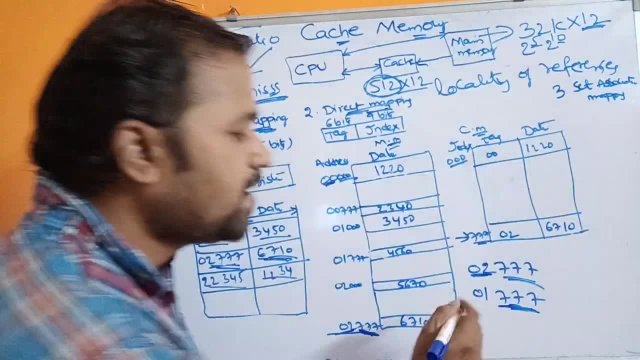 So this 777 is useful in order to access the cache memory. But here, what is the tag here? 0, 1.. But here, what is the tag here? 0, 2.. So these two are not matching here. 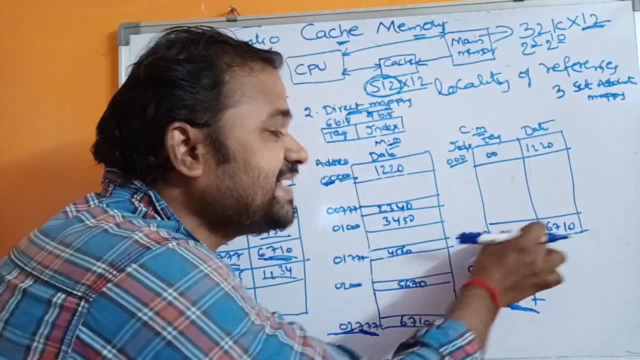 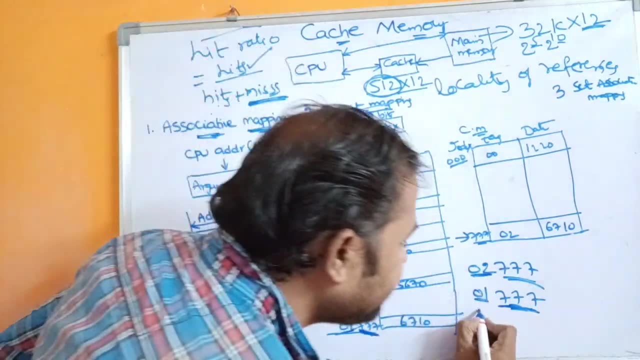 Why? Because here the problem. The problem is in an index address. it is not possible to store multiple tags, So multiple votes are not stored here. So if let us assume that we have one more, request 0,, 4,, 777.. 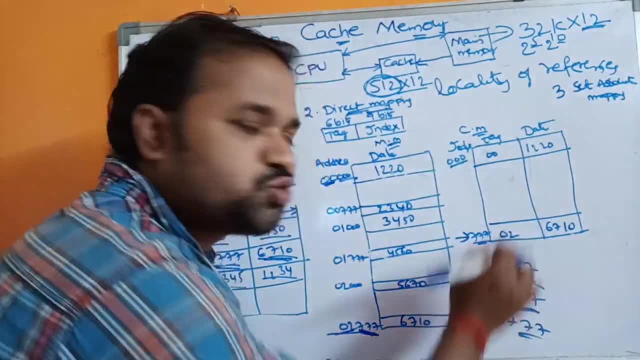 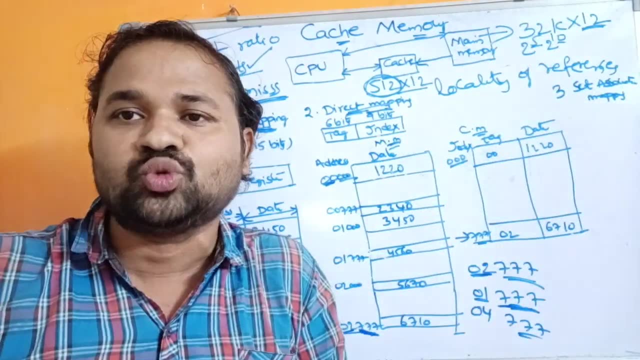 So 777 is the index address, But 0 to 0,, 4, these two are not matching. So what is happening here? Several times misses are there. So if there is a miss, then what we have to do? 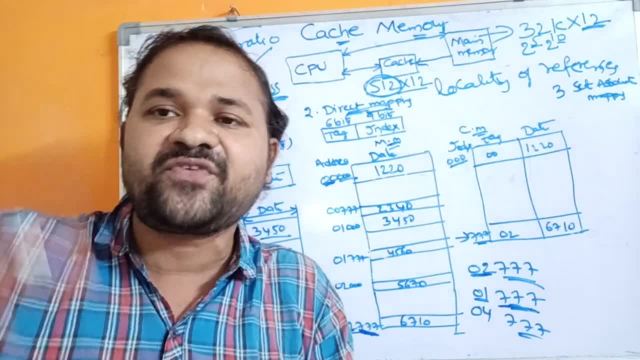 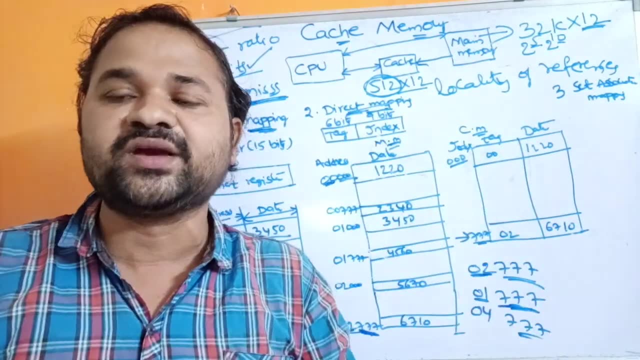 That vote is not present in the cache, So that vote should be transferred from main memory to the cache memory. So several times We are transferring the data from main memory to the cache memory, So the performance of the hit ratio will decrease drastically. 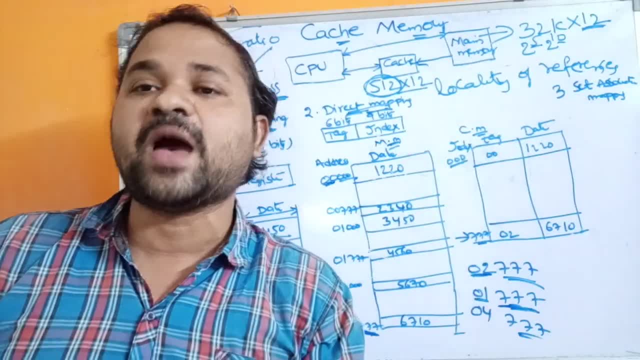 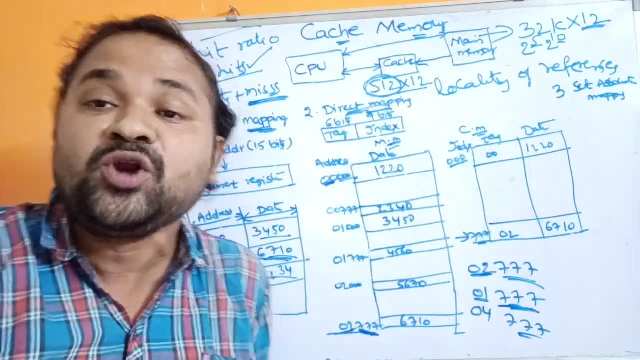 We can overcome this problem with the help of set associative mapping. The major advantage of the set associative mapping is: in a single index we can store multiple votes. So this is the first vote here. So if we want, we can store second vote also here. 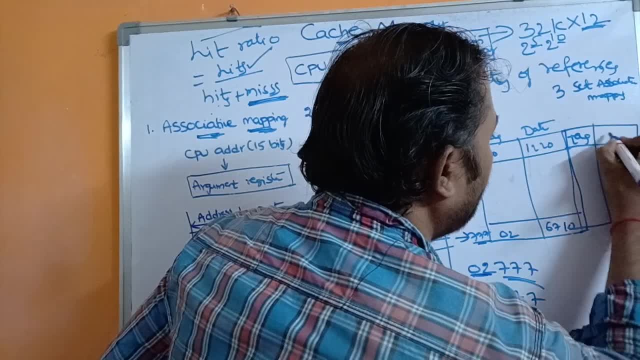 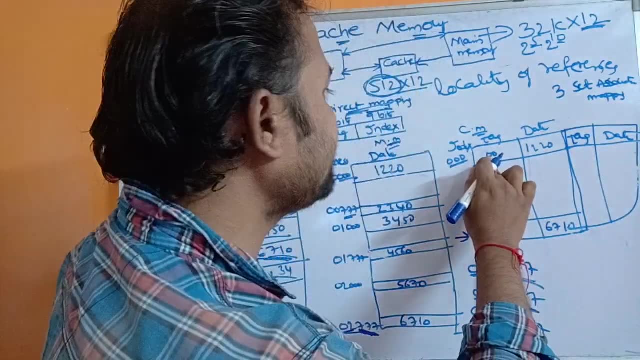 Let. this is nothing but second vote tag. So second vote data. Okay, Let here. Let the second vote tag is second vote. this is nothing but here. What is the tag? 0, 0 is the tag here. 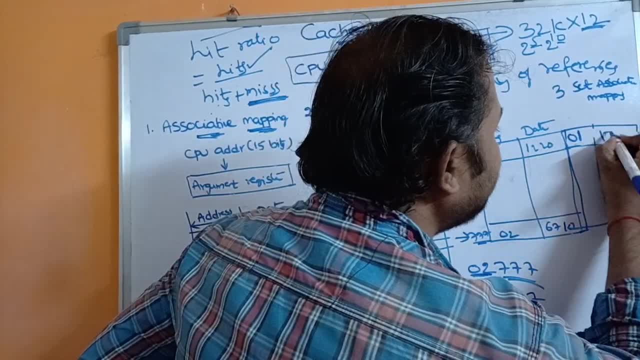 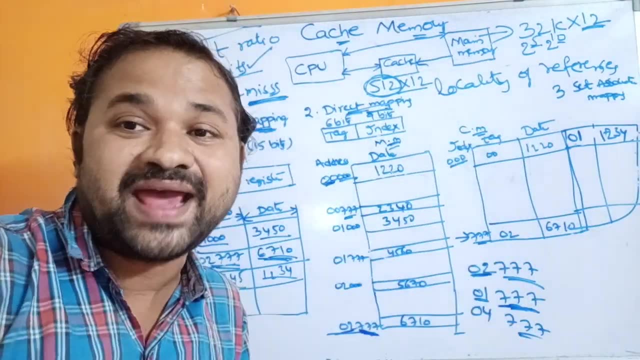 Let here the tag is 0,, 1.. 0,, 1. Let the data is 1,, 2,, 3,, 4. So likewise here also. So in each index address we can store multiple tags, multiple votes. 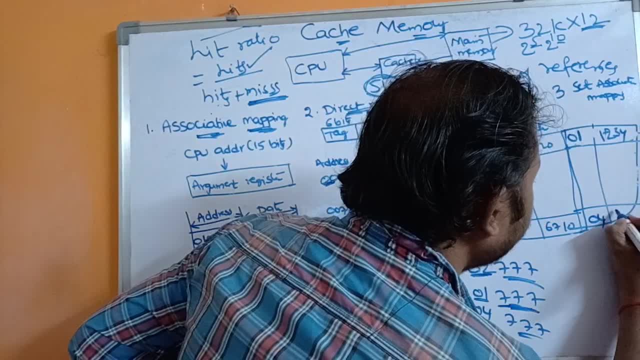 So let here the tag is 0, 4.. And the vote is 4, 5, 6, 7.. So let us assume that we want to access this address: 0, 4, 3, 4, 7.. 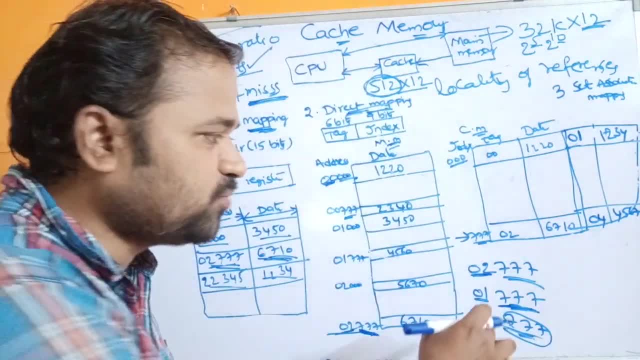 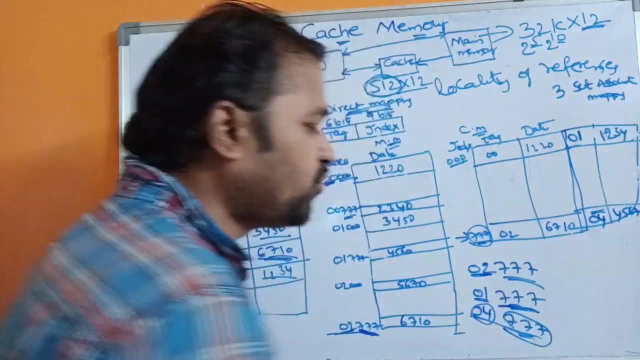 So this index address is useful in order to access the cache memory. So this 777 is useful. Next, what is the tag here? 0, 4.. Here we do not have 0, 2. But here we have 0, 4.. 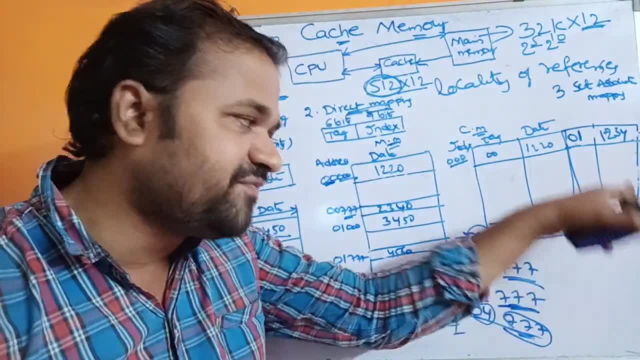 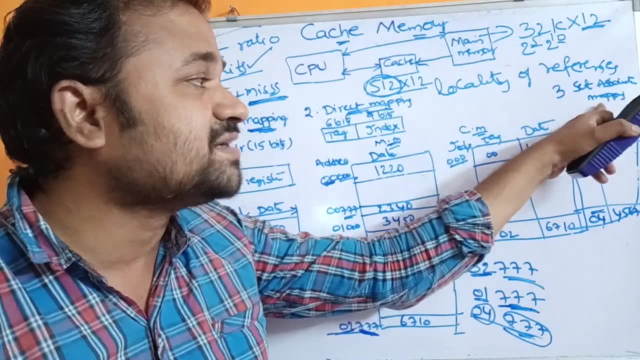 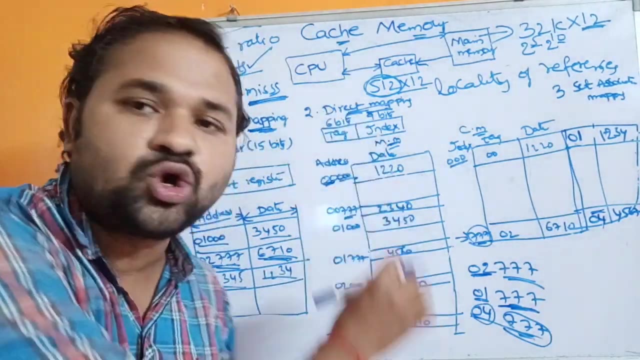 So set is found. Match is found. So cache memory allocates this vote to the CPU. So CPU executes that vote. So the major advantage of the set associative when compared with direct mapping is in direct mapping in each index address we can store only one tag. 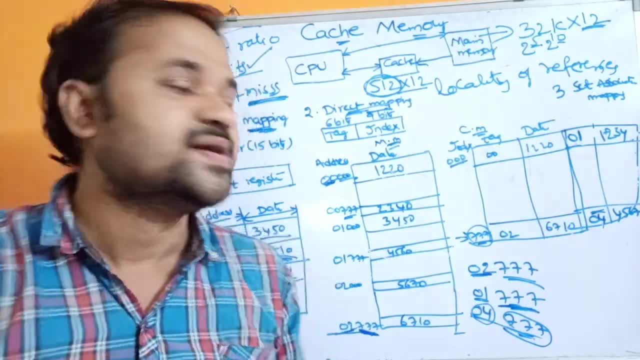 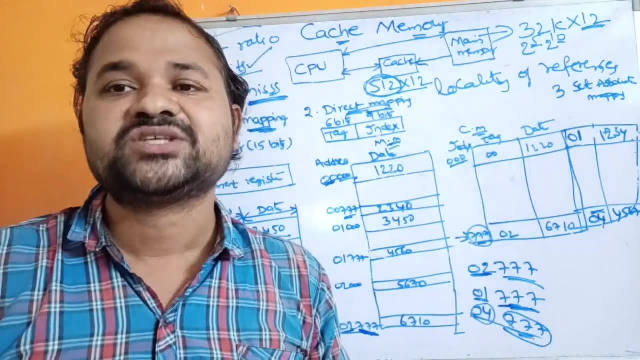 That That means each index address can store only one vote only, Whereas with the help of set associative mapping at each index address, we can store multiple tags. So this is about what is cache memory and what are the various mapping functions. 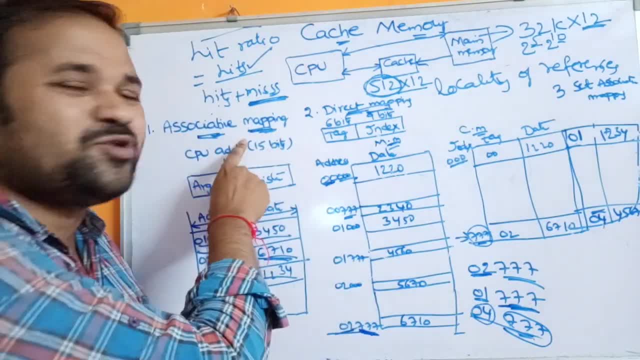 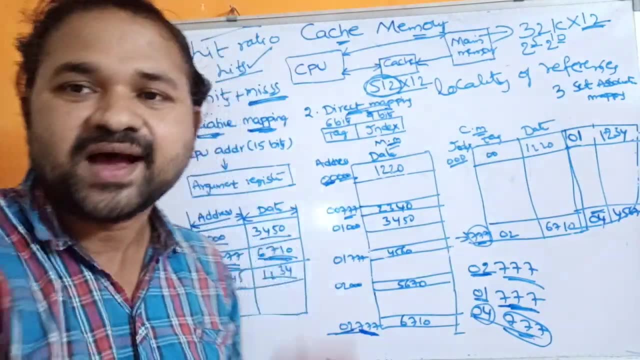 So totally. there are three mapping functions: Direct, associative mapping. Associative mapping is very, very expensive. We will discuss more about associative memory in the future videos. Associative mapping is very, very expensive. We can overcome the problem with direct mapping. 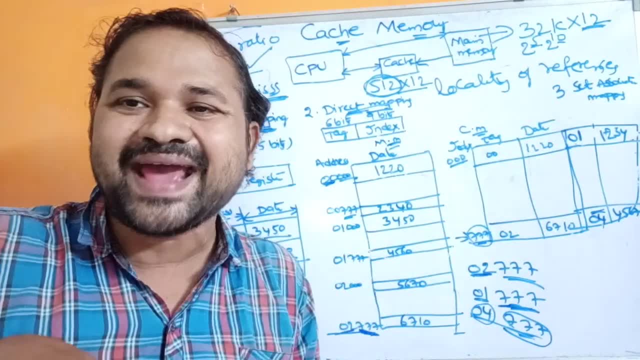 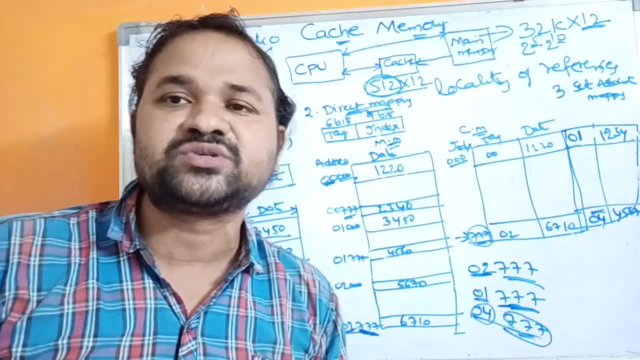 But the problem with direct mapping is each index address can store only one tag, So there is a possibility that hit ratio may decrease drastically. So we can overcome that problem with the help of set associative mapping. 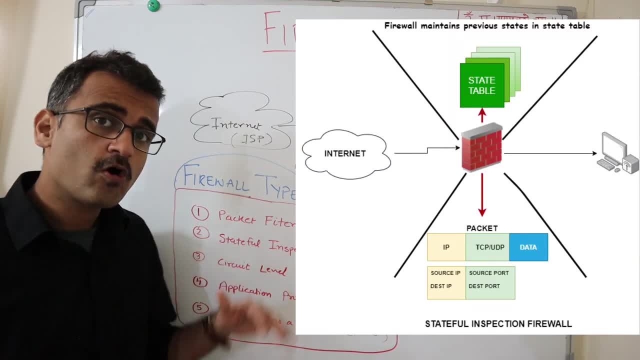 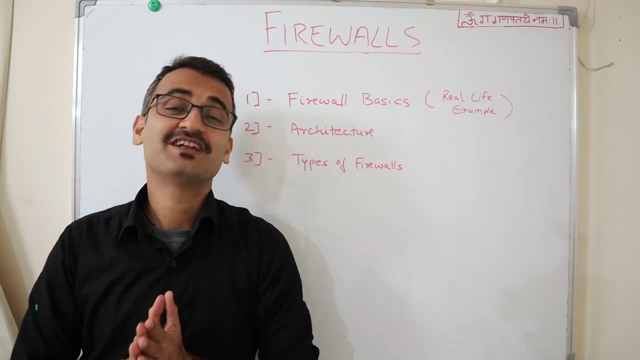 of any particular traffic which is coming in. so it is keeping a track of previous packets which has gone in and the new packet which is coming in. hello friends, welcome to itk funday, your own channel, where we make it interesting for everyone, and in this video we'll understand about firewall. 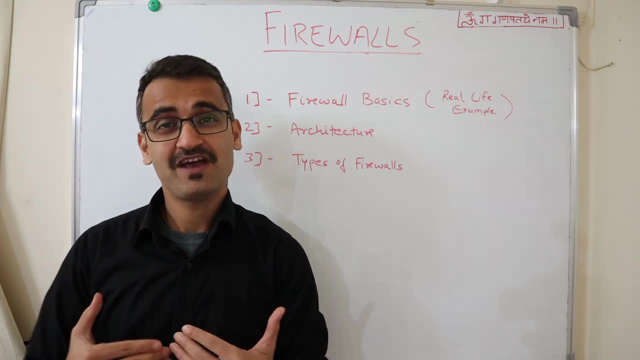 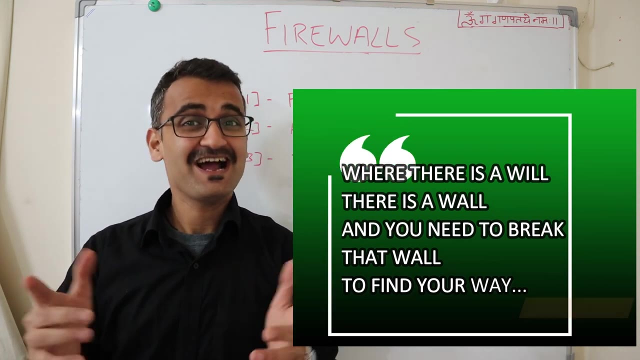 there's a famous saying: where there is a will, there is a way. but if you ask me, i often say that where there is a will, there is a wall, and you need to break that wall to find your way, and that wall in networking is none other than a firewall. so if someone wants to get into your 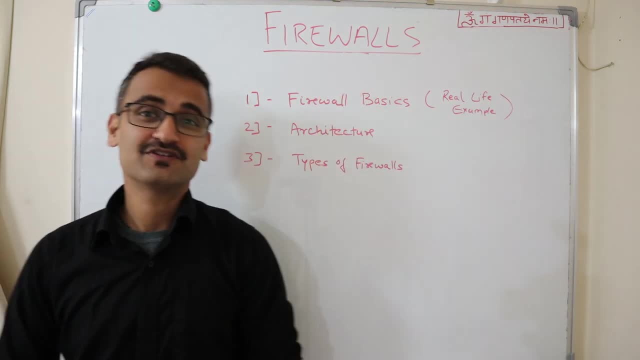 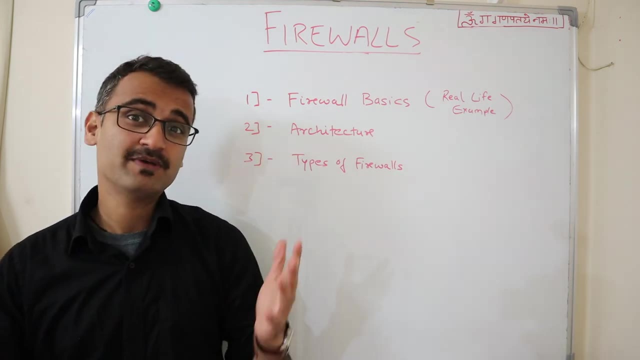 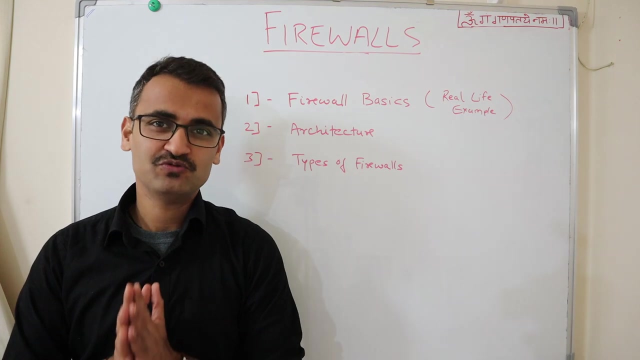 network, he or she needs to break this firewall at first place. so in this video we'll understand what is a firewall, with a basic real life example. we'll understand the basic architecture of how firewall works and at the end we'll also understand about some basic types of firewall which we use. so 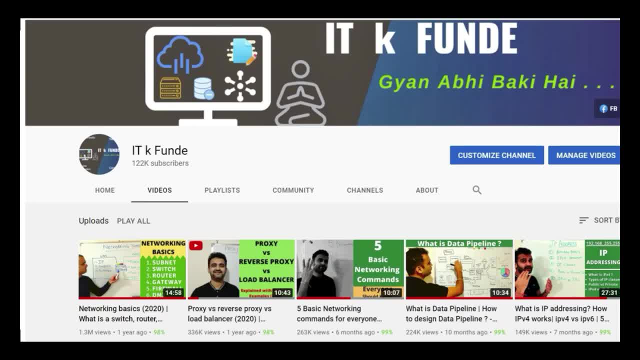 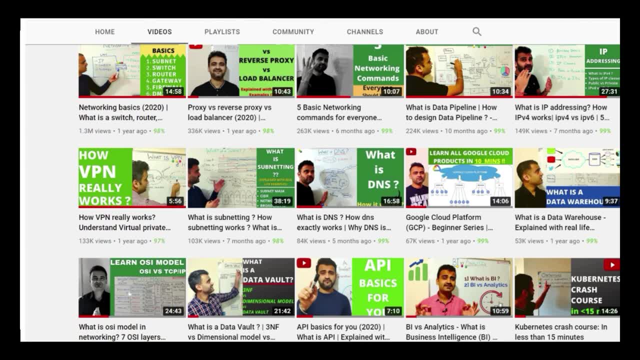 without further ado, let's get started. thank you, friends. if you're new to itk funday channel, we make it interesting for everyone and we'll see you in the next video. bye, bye one. be it it or non-it, we discuss all the latest tools and technologies, products, productivity, hacks. 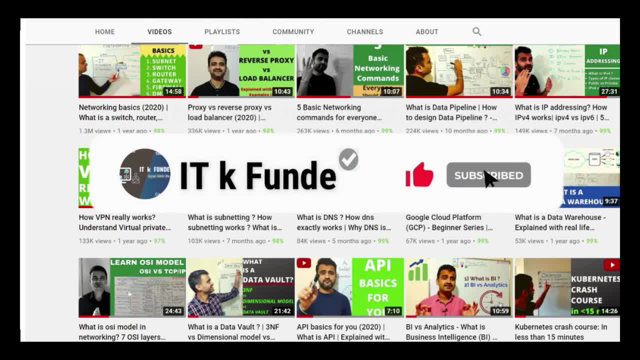 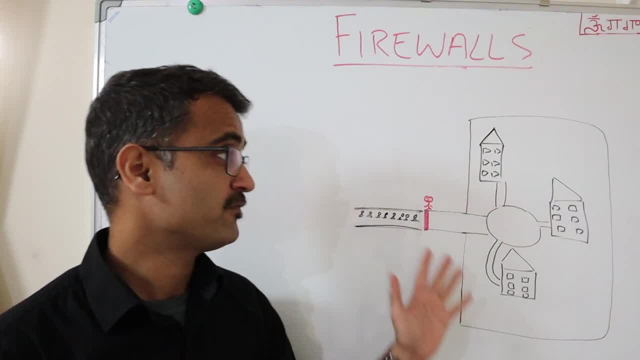 and carrier tips on this channel. so if you are new and if you like the content, do consider subscribing. thank you. so, friends, if we take a real life example, uh, you can take an example of a housing society where we have three different buildings and people staying in their own apartments.